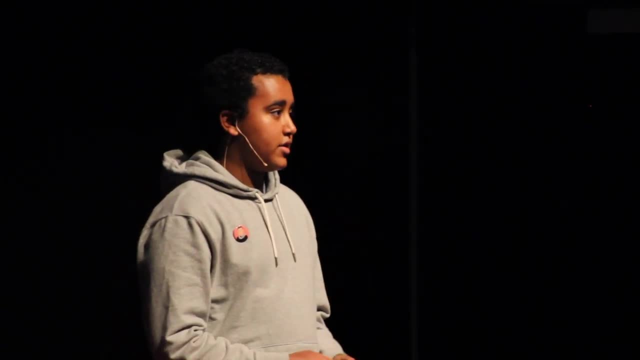 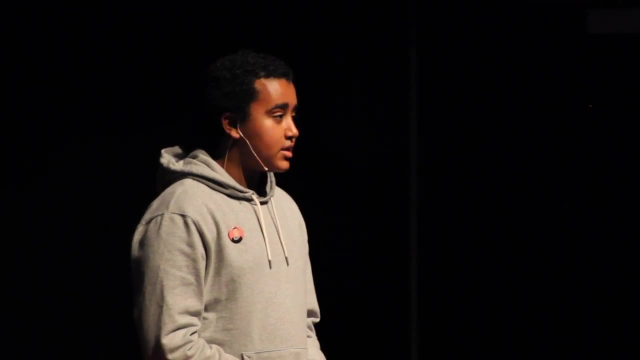 Furthermore, both of my parents grew up during the communist regime in Ethiopia, known as the Derg, where they didn't have any say in how their government functioned. It is for both of these reasons that I've spent most of my free time focused on learning how I 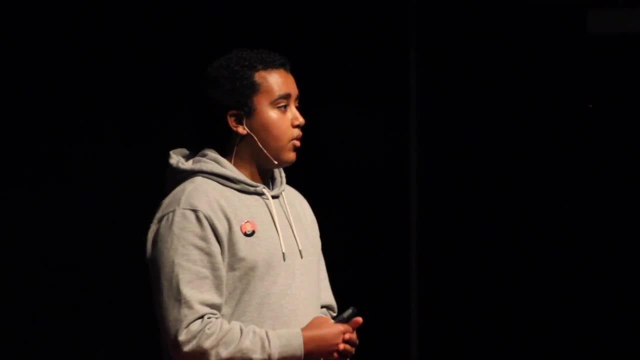 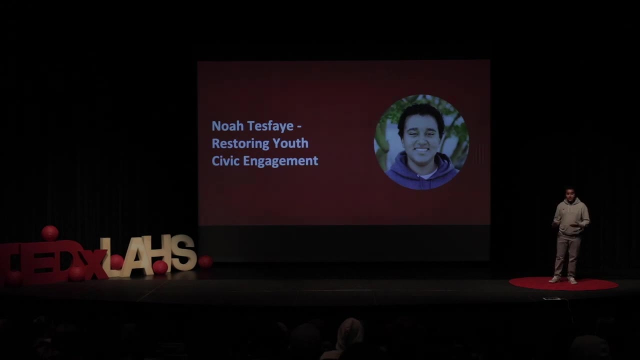 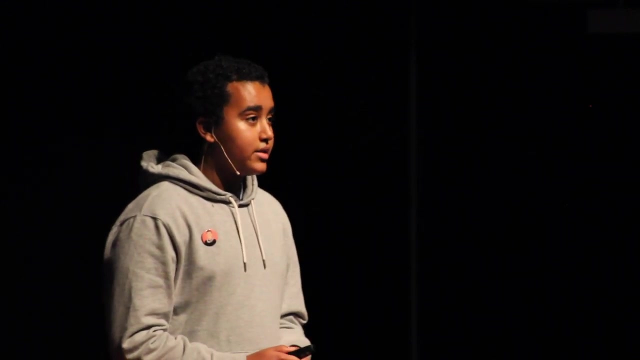 could better educate myself and ensure that I could become a more empowered voter in this country. However, I, along with millions of other Americans across the country, are in the minority. Just 31% of Americans age 18 through 29 voted during the 2018 midterms. 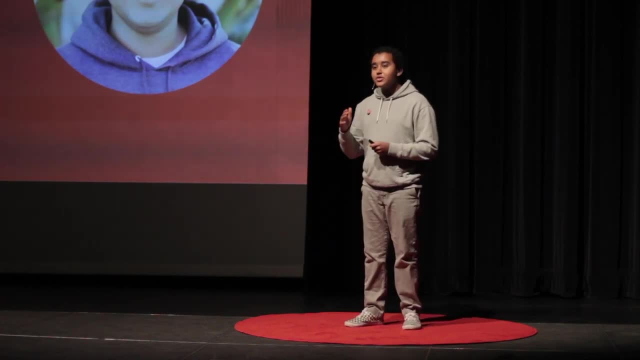 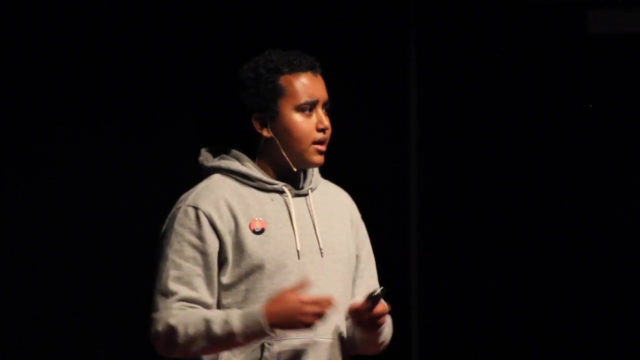 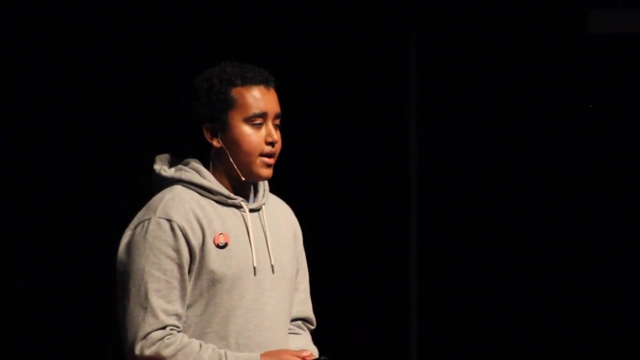 Furthermore, just 1 in 3 Americans can pass a citizenship test. 1 in 3.. That's compared to the 91% immigrant pass rate of that same test. Much of this ultimately comes down to civics education. During the 1960s and the Vietnam War was going on and most of the 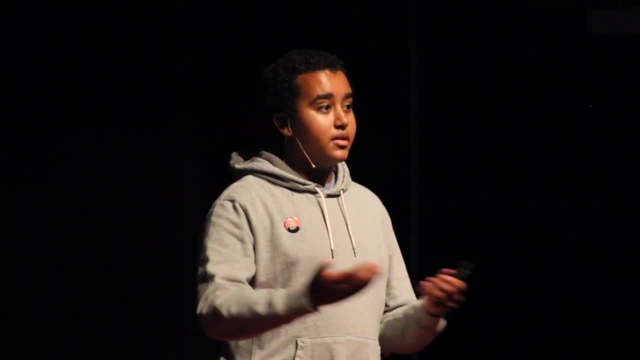 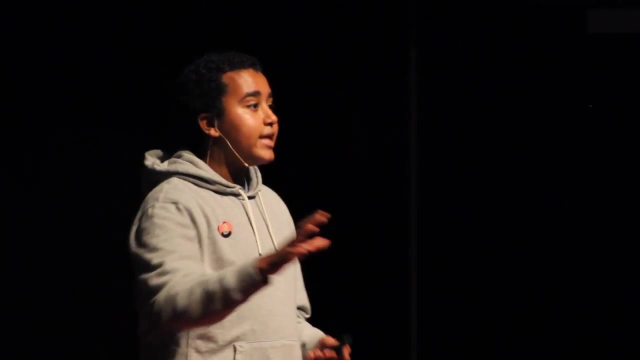 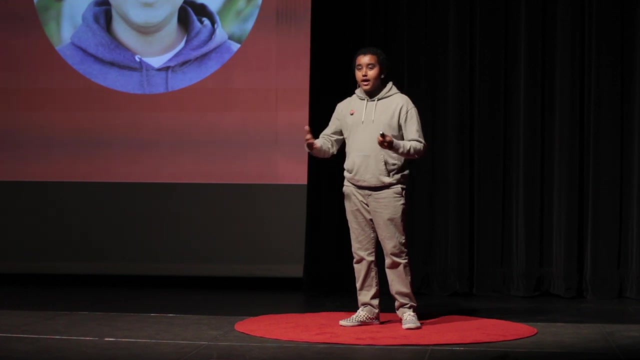 federal government thought it would be a good idea to dumb down civics and depoliticize the classroom. Since then, we've seen voter turnout rates for young people go from around 50% down to the 31% we see today. Much of this comes from a lack of strong civics education. 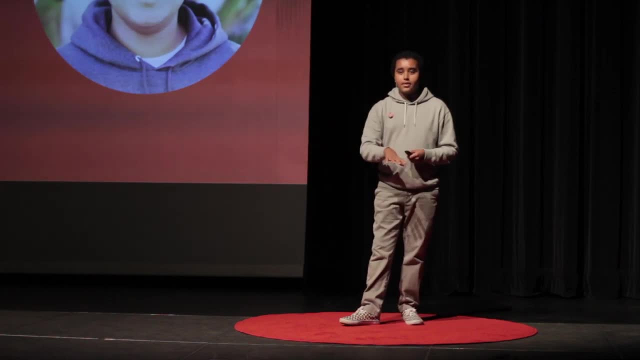 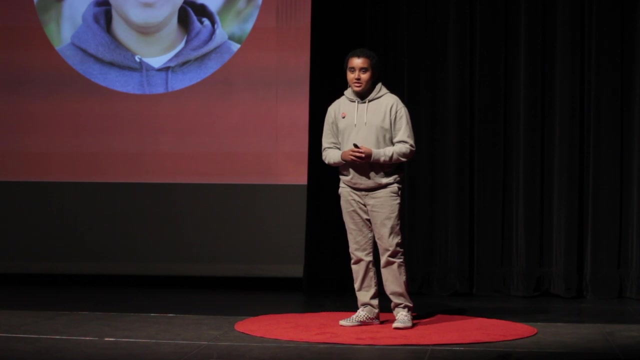 That is where, in many parts, our school, Los Altos, is a problem. See, we only have three options for civics education: It's AP Gov, regular civics and global connections. However, our education requirement is only one semester during senior year. That is a grave problem. 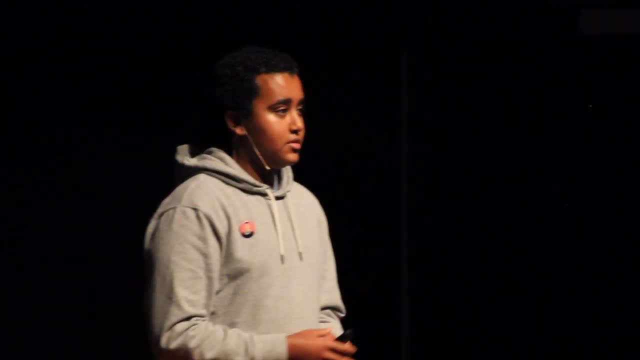 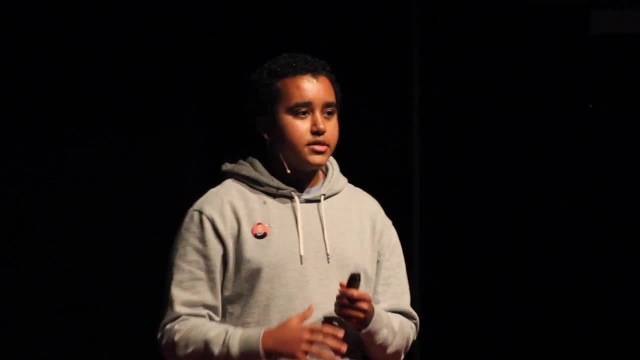 If we can further go back and look at some of the research that's been done. a Tufts University research center spent years looking at civics education, analyzing different classroom settings and different ways in which we could further empower our voters, And they found 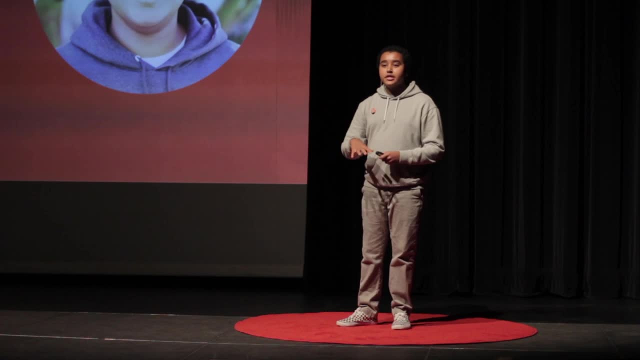 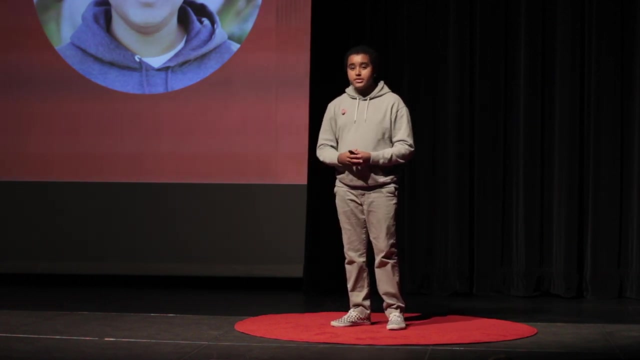 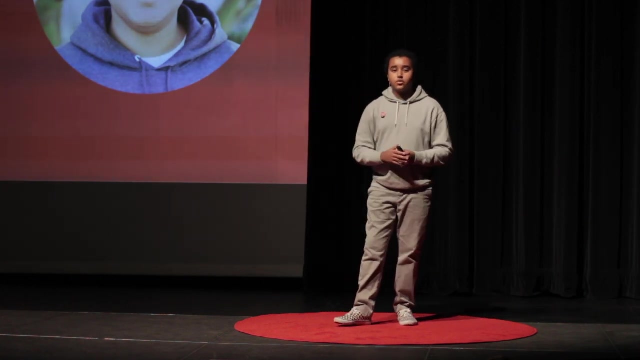 one thing That if we started civics education in middle or even elementary school, we'd get a higher voter turnout. That would prevent any sort of issues that we see with the 31% voter turnout rate and only 23% of Americans that took the middle school civics education national exam passed or exceeded. 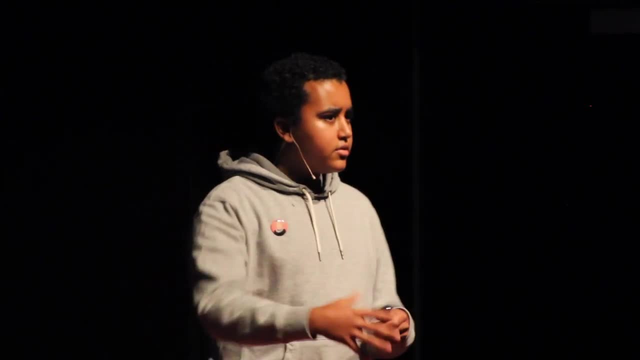 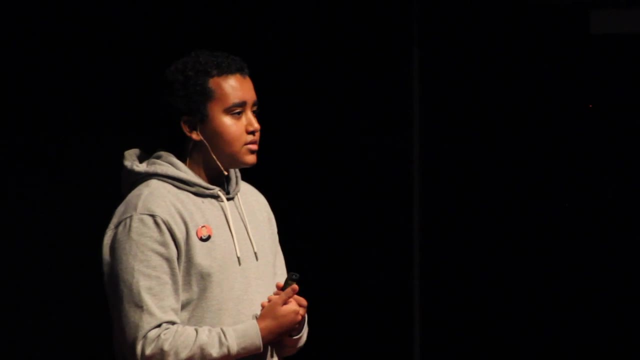 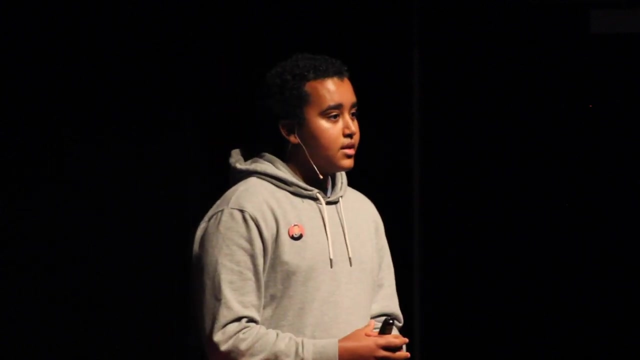 standards And if we further implement those discussions in the classroom. that's how we can further our goals Right Civics education is by far the most important class for any citizen of this country, for one reason: It allows you to understand how we function as a society. It allows you to understand 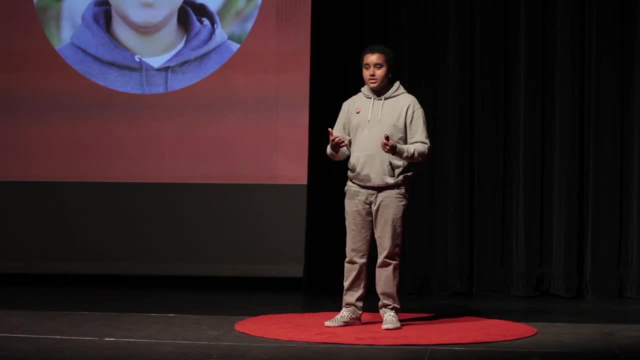 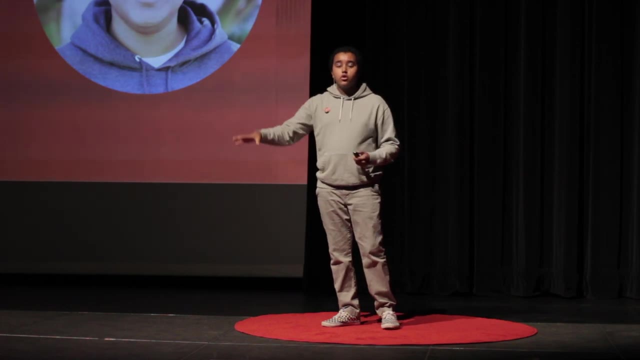 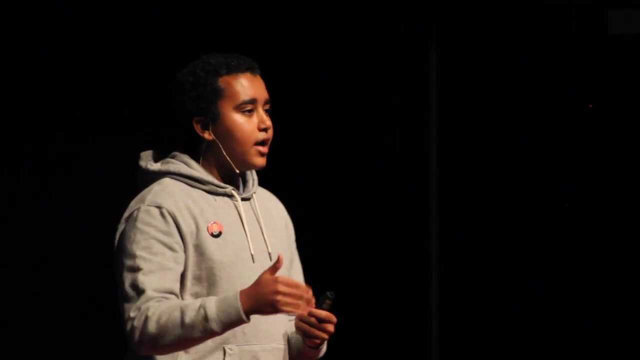 the different branches of government, the intricacies that go within policymaking Congress. It allows you to understand that states, for example, have more control over your educational requirements and not the federal government Right. It allows you to understand that it's not just about how laws are implemented. 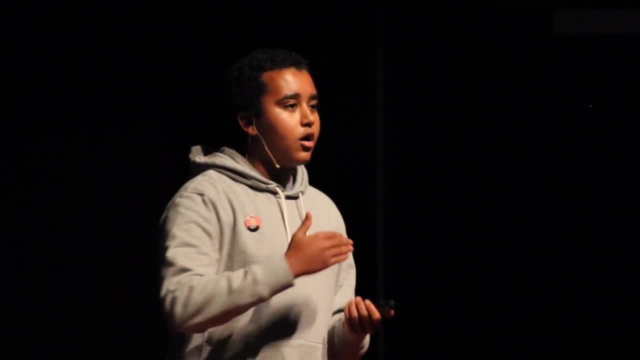 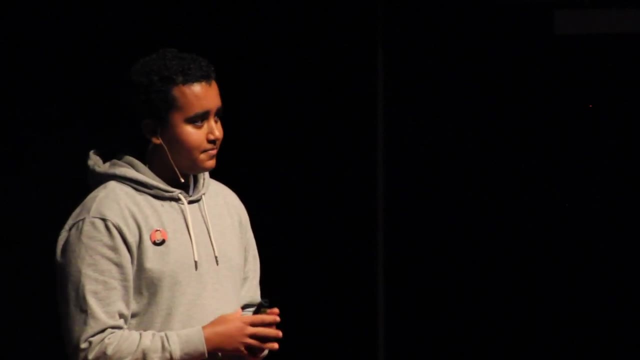 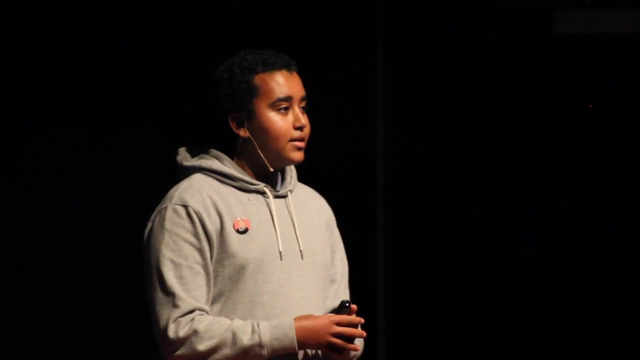 but it's about how the public receives them and to what extent they are enforced by our local governments. This is why civics education is important. Now there's a common misconception and complaint by adults that by increasing more discussions about politics in our classrooms, 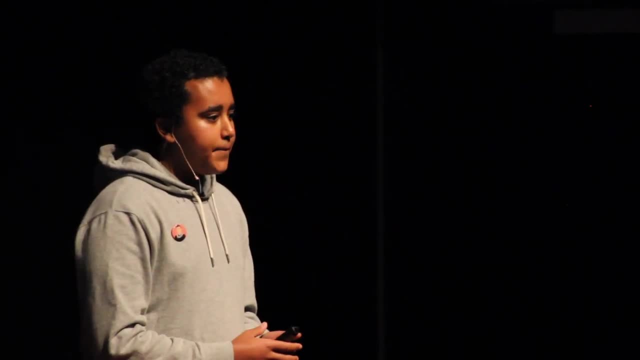 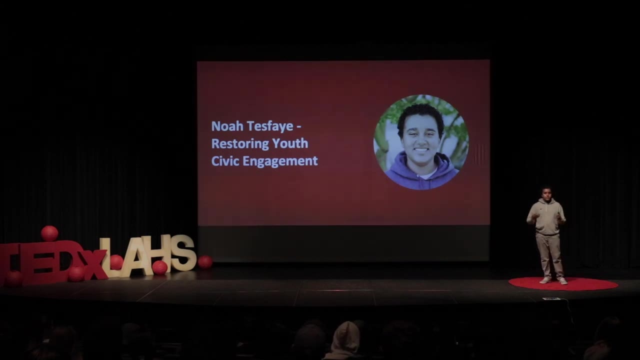 we'll have an over-politicized classroom. But I'll ask you this: what good is education as a whole if we cannot have those conversations amongst our peers in a classroom discussion in which we can be challenged on our ideas and not have to stick to the status quo? 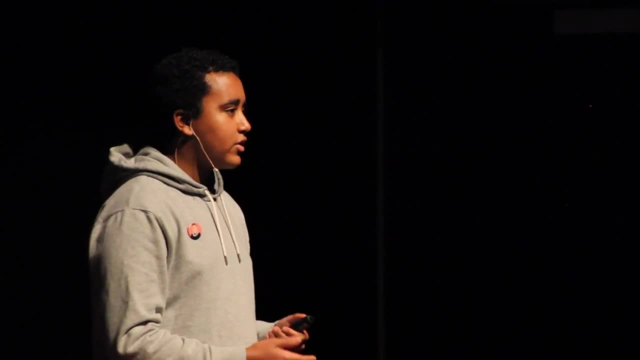 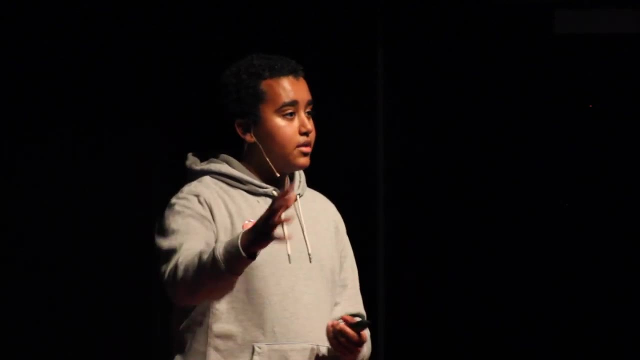 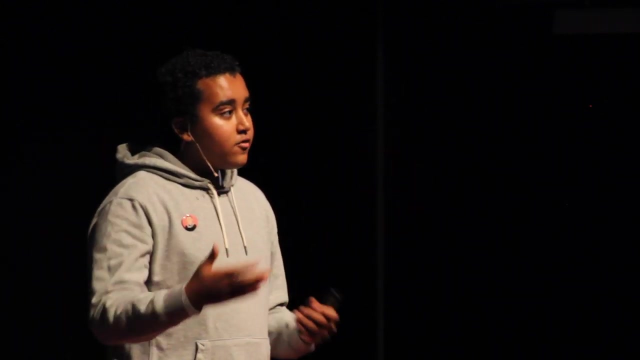 Furthermore, adults could really do more to further our academic goals as well. How are we supposed to be more educated and influential in the political system when people are calling us self-centered or too fringe-right or too socialist-left, If we can't have that discussion inside a classroom? 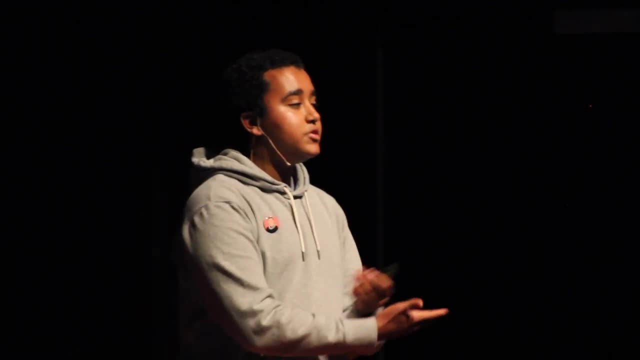 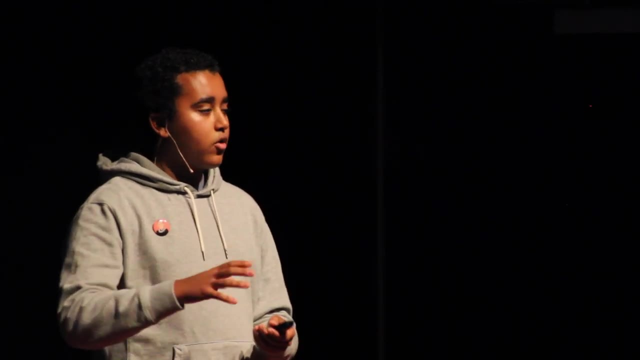 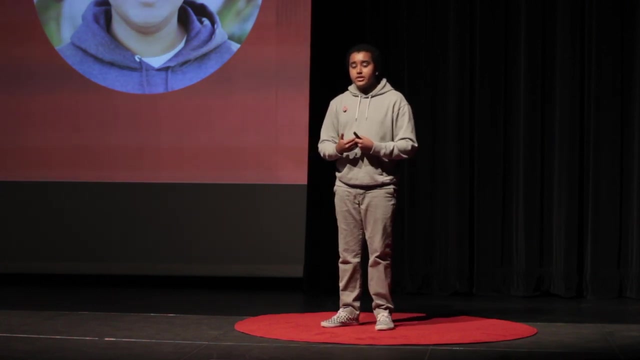 with a teacher who's ready to help answer any questions, give an objective layout as to how politics works. that's when we can finally be able to get closer to a more empowered voting electorate. Look, I'm not going to say that civics education is a partisan issue. 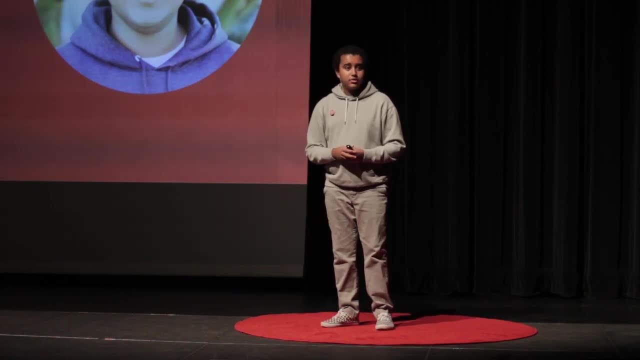 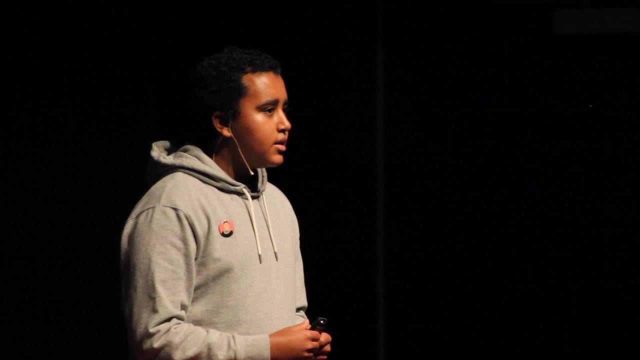 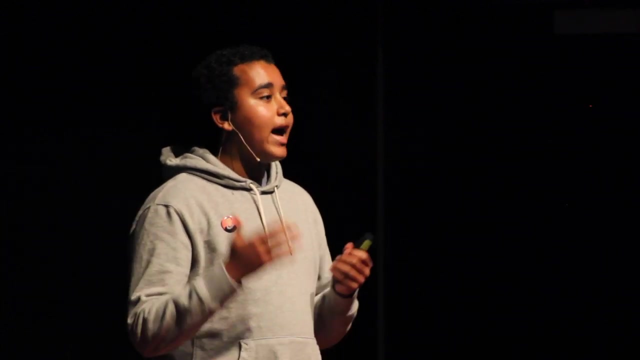 because it really isn't. It's an American issue. Ensuring that people get registered and understand how to vote is not a partisan issue. It's an American issue. If we want to have the best Republican democracy that we can, we have to get out to vote. 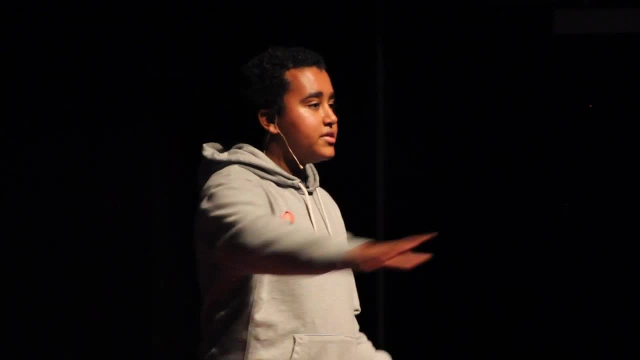 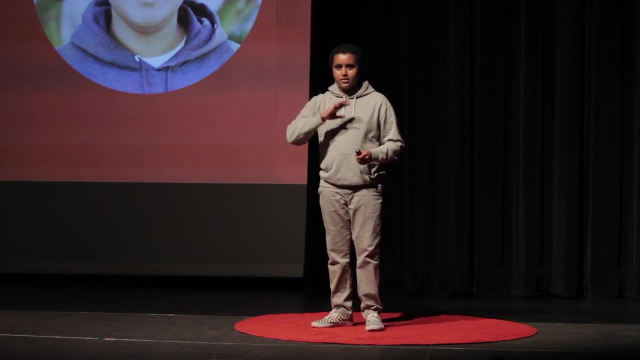 That's the only way our society can truly represent the voices of the millions across this country. Now, last Thursday, I had the chance to attend a talk at the Flint Center where James Comey was giving a speech, and, irrespective of what you may think about James Comey, 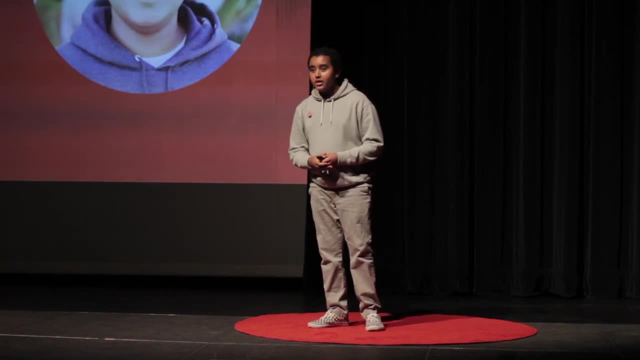 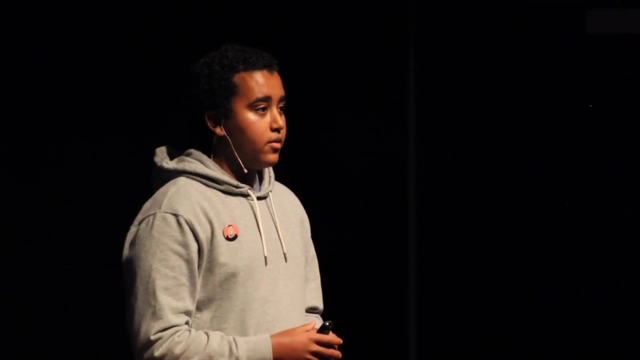 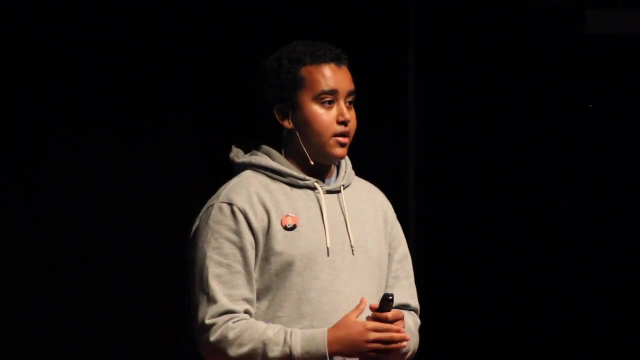 I got the chance to ask him this question. If you were to convince a high school student how to vote or why they should vote, what would you say? He told me this: that we would not have any say in our democracy as a whole. 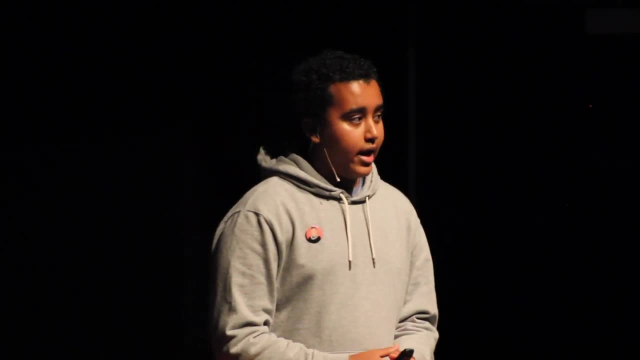 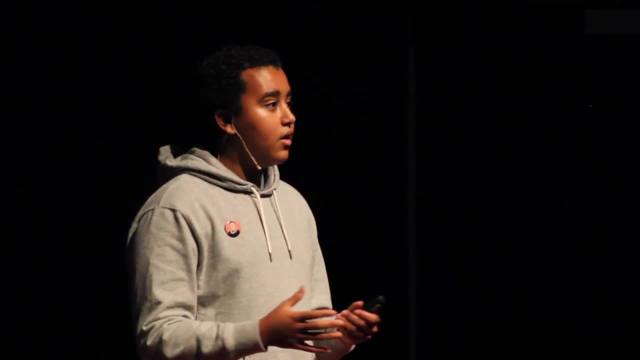 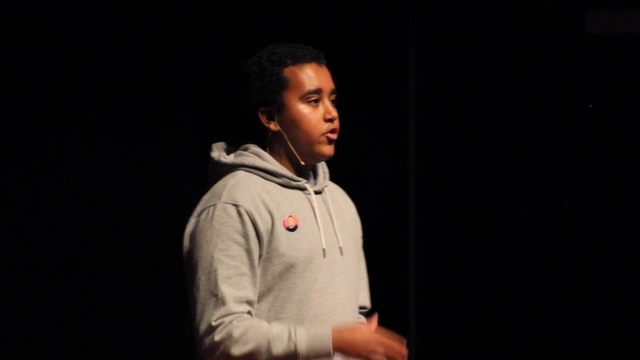 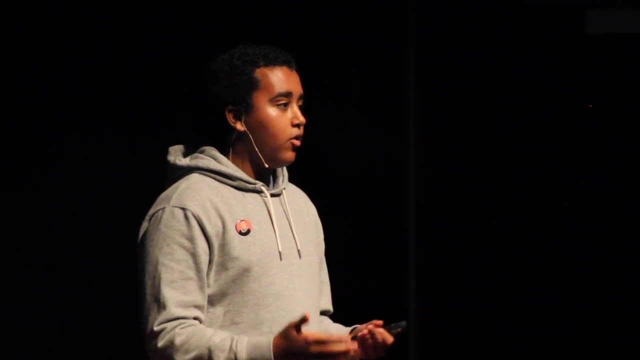 he fails to focus on the biggest issue of them all: That how are we supposed to actually ensure that people get out to vote, that they're active in politics, that they know who, which candidates and which policies are on their ballot, if they are not educated in how we vote? 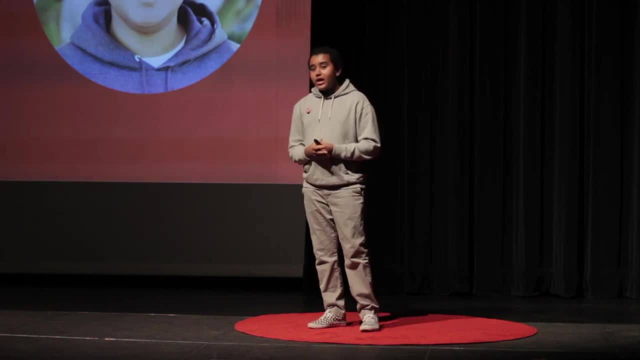 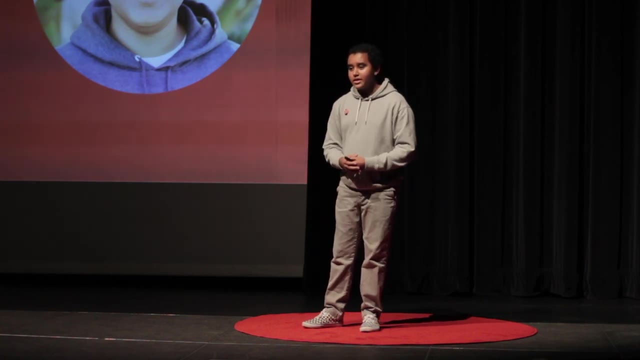 So, even though I may not be the most politically active citizen in this country, I think that there is room for us to vote. So, even though I may not be the most politically active citizen in this country, this room or even in this school, I've sought out ways in which I can further understand. 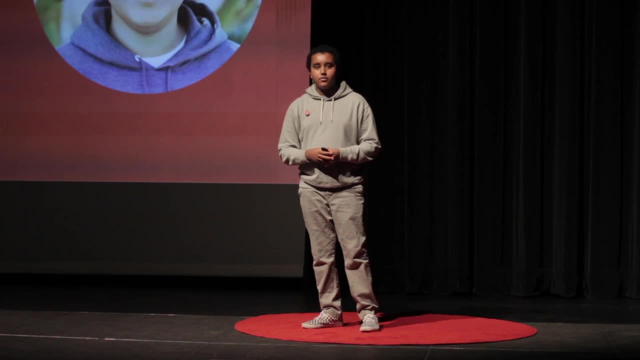 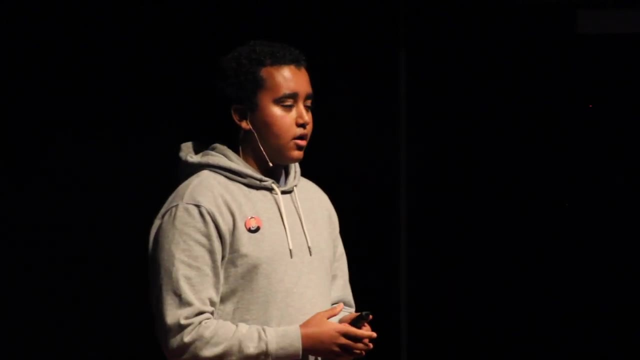 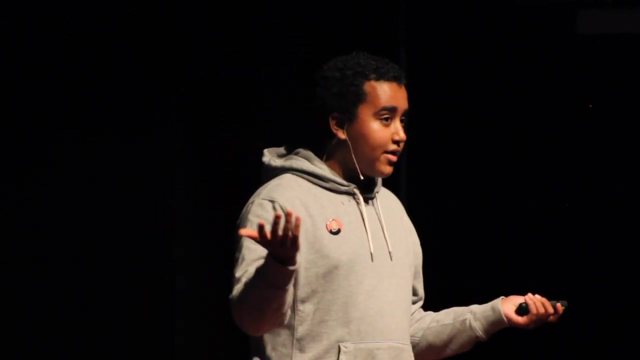 this society. through my writing as a journalist, I've sought methods in which I could try to bring a new perspective, to share a new voice as to how we could further impact our community, whether that's covering the local city council elections, to discussing our March for Our Lives protest last year and understanding 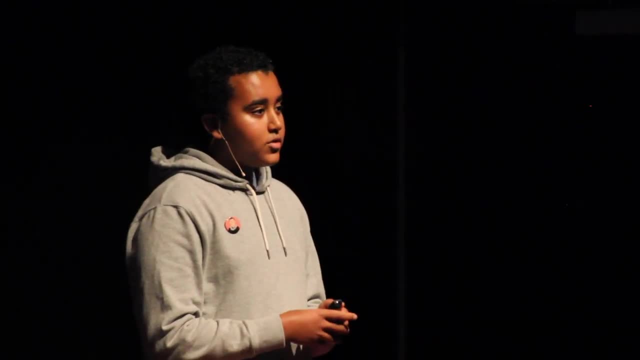 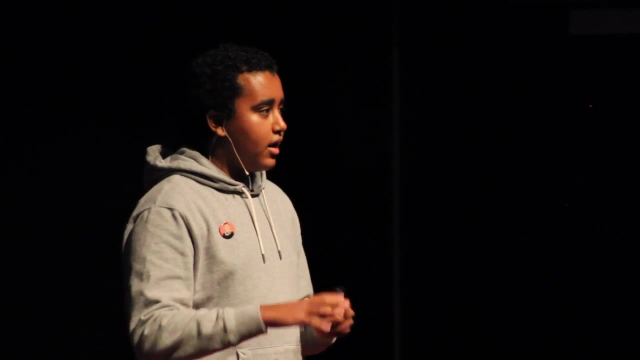 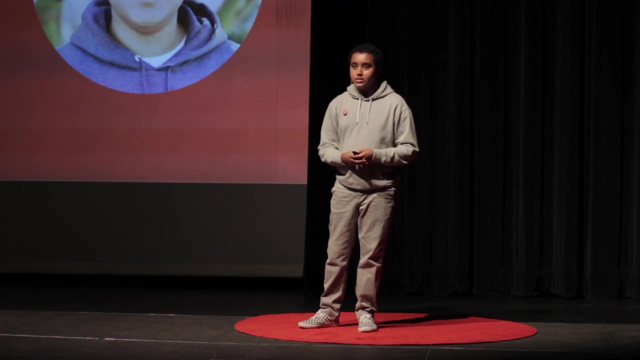 student protest dynamics. I am slowly but surely trying to ensure that I can be a more active and productive member of this community and of this country. Now I know many of you may be thinking: well, what can we do? What can you do?